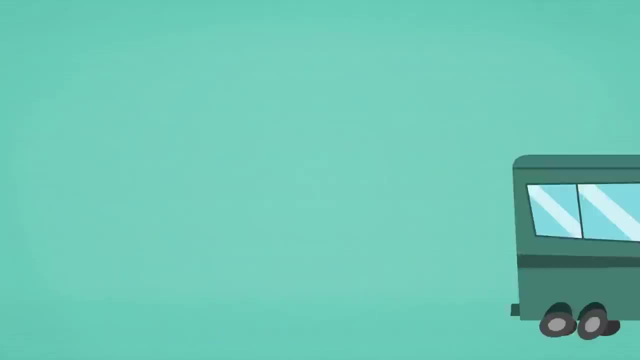 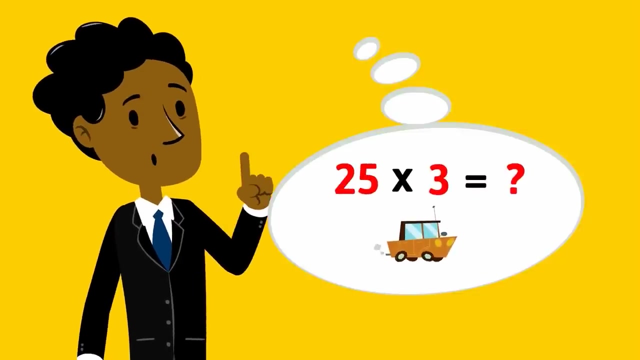 words, its speed is changing. Now that we have a more realistic problem, how can we determine how far the car will travel in 3 hours? The answer lies in calculus, and it's just one example where we want to be able to mathematically. 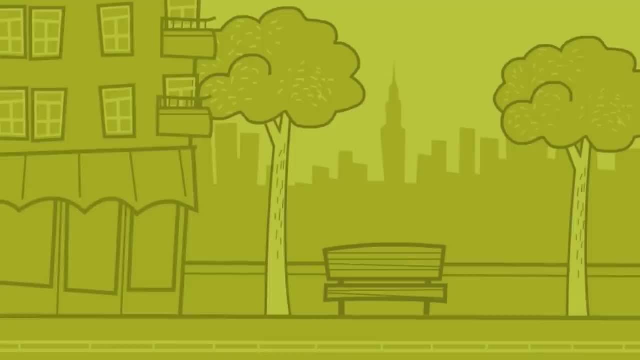 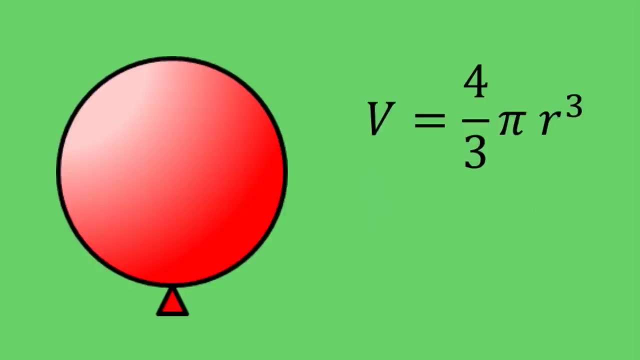 calculate the speed of the car. Here is another quick example. If I want to model the volume of a balloon, you might assume that it's approximately a sphere- And then use the formula of: volume equals 4 thirds pi times the radius cubed. This shows that the volume of a balloon is related to its 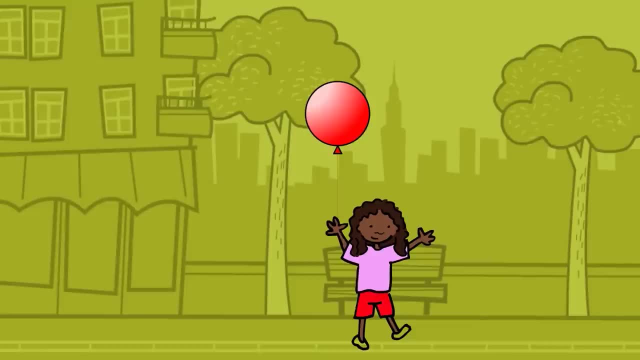 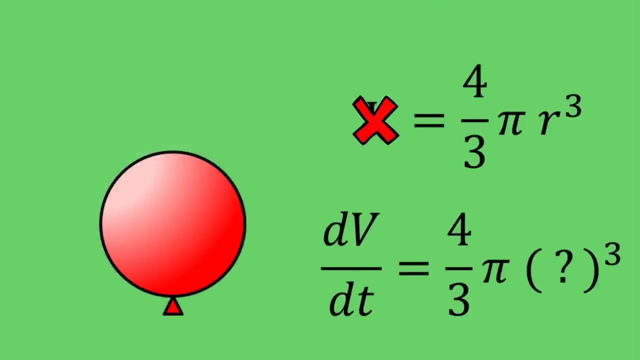 radius. Now, when I start to let air out, things start to change. The volume all of a sudden starts decreasing And so does the radius. But how are these changing quantities related to one another? now, What is the formula for this change? Again, the answer lies in calculus. 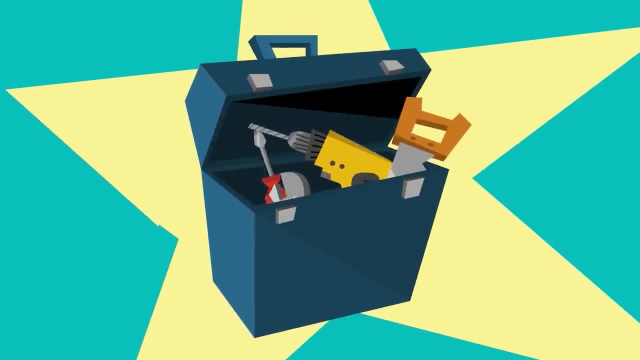 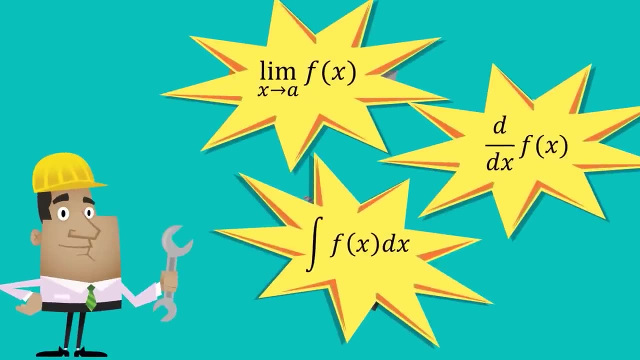 So, in order to tackle the problem of changing quantities, calculus picks up 3 powerful tools. These tools are limits, derivatives and integrals. Now, there are many other things you'll learn in calculus, but these 3 things are the most essential. Because of this, you'll want to. 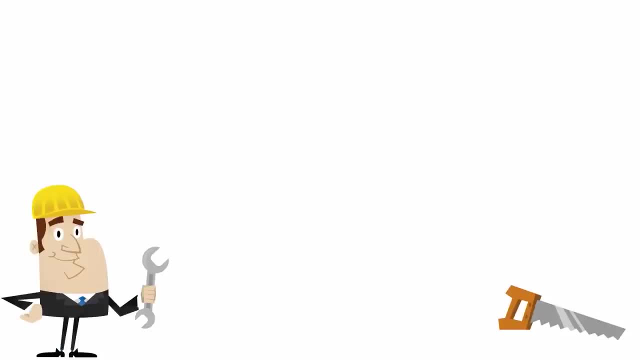 spend as much time with them as possible. So let's take a look at one of these. Limits are the tools we use for precisely describing how a function approaches a value. Derivatives are the tools we use for describing how a function changes, And integrals give. 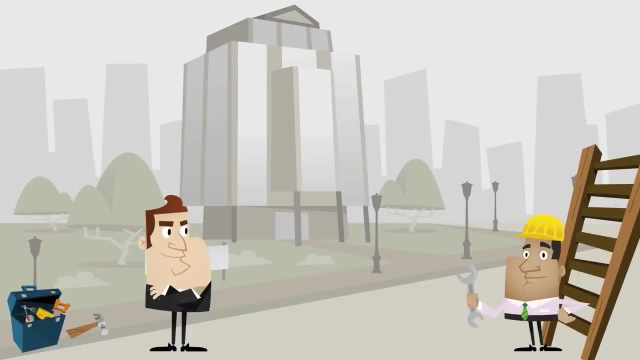 us the area underneath the curve of a function. Using limits, derivatives and integrals, calculus can solve a variety of different problems, like where to sit in a theater for optimal viewing or even how to make the perfect soup can. One of the most fascinating aspects of calculus is how all of these tools can. 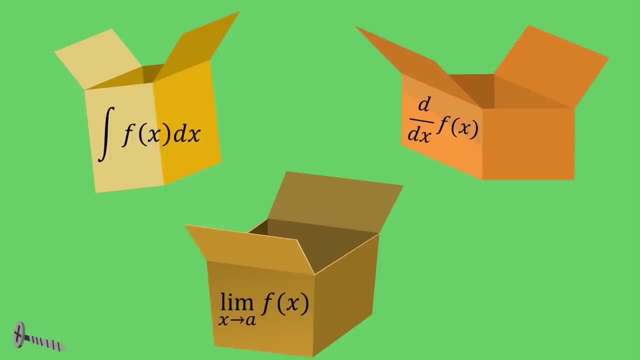 actually be related to one another, Even though they may seem completely different. derivatives are built from limits, and integrals can be viewed as the inverse of a derivative. Of course, you'll learn all of this when we start to dig deeper into the subject. 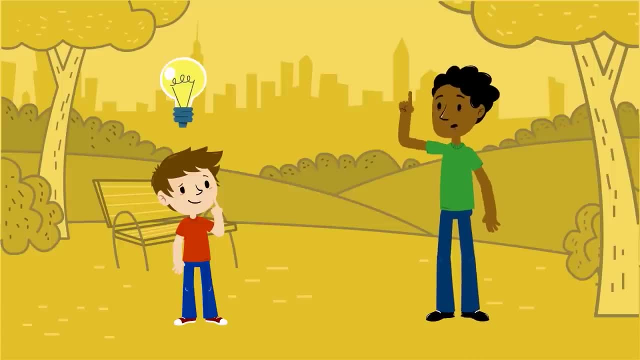 For now know that calculus can be difficult, with many new ideas, terms and procedures, But we learn it because it provides a better way to describe the world around us, especially when it comes to change. Hopefully that gives you a better idea of what.